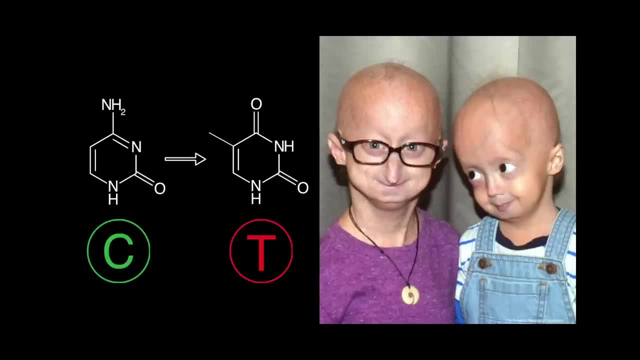 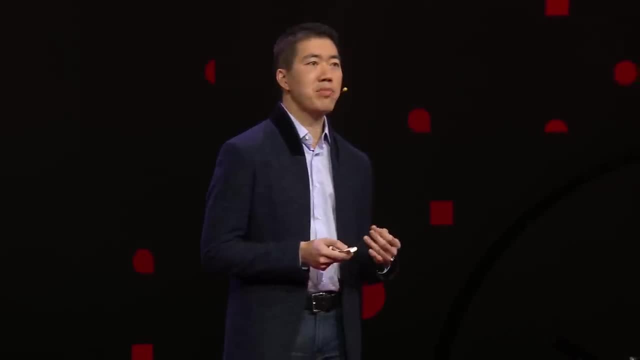 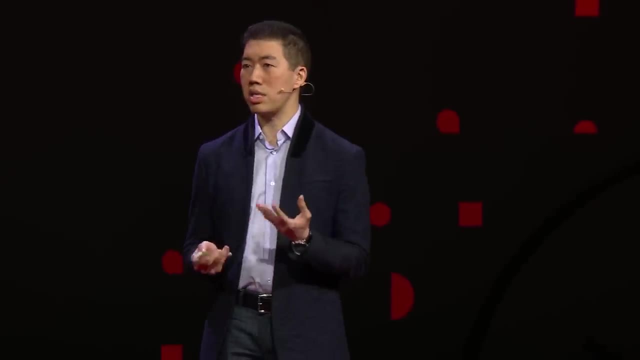 with the devastating consequence that these wonderful, bright kids age very rapidly and pass away by about age 14.. Throughout the history of medicine we have not had a way to efficiently correct point mutations in living systems, to change that disease-causing T back into a C. 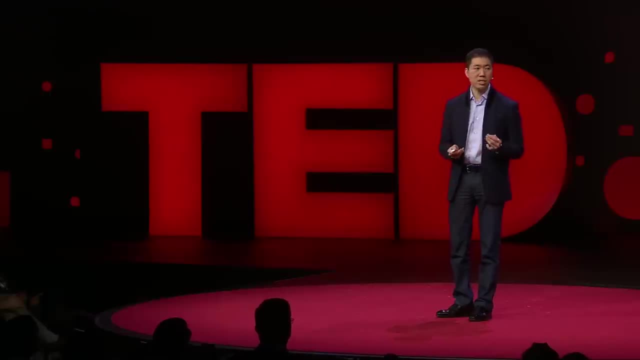 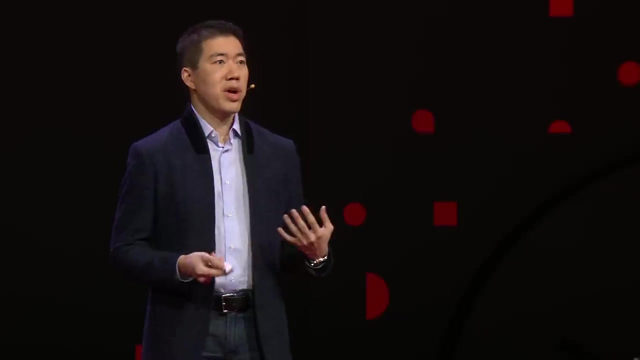 Perhaps until now, because my laboratory recently succeeded in developing a system that could correct point mutations, And I think that's why we're developing such a capability, which we call base editing. The story of how we developed base editing actually begins three billion years ago. 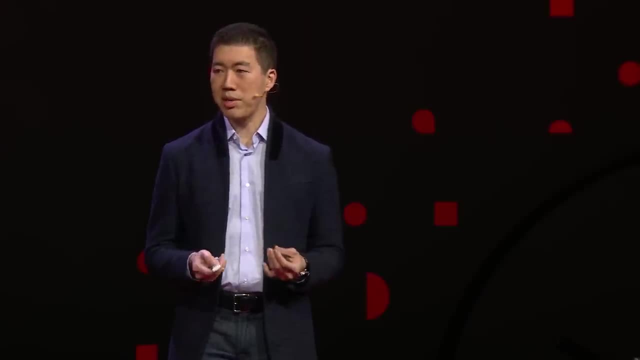 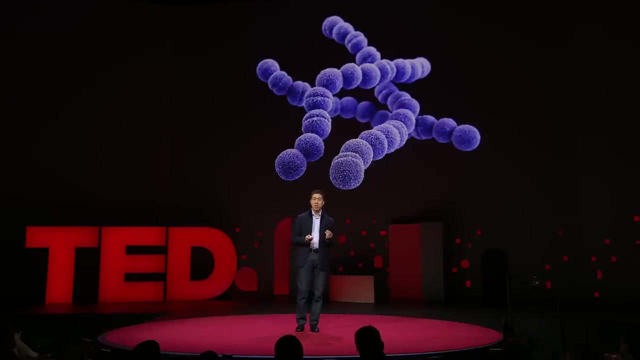 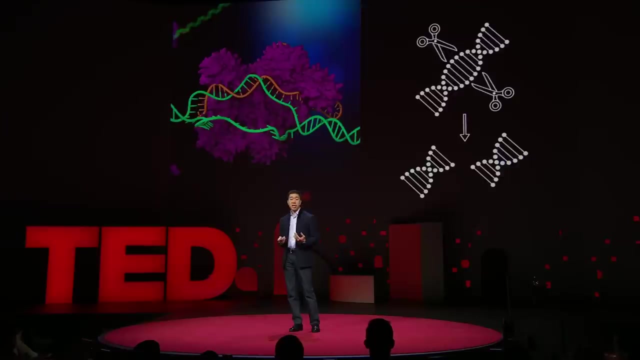 We think of bacteria as sources of infection, but bacteria themselves are also prone to being infected, in particular by viruses. So about three billion years ago, bacteria evolved a defense mechanism to fight viral infection. That defense mechanism is now better known as cryptocoryne. 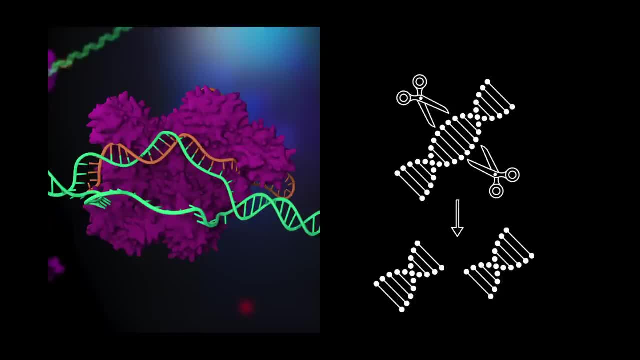 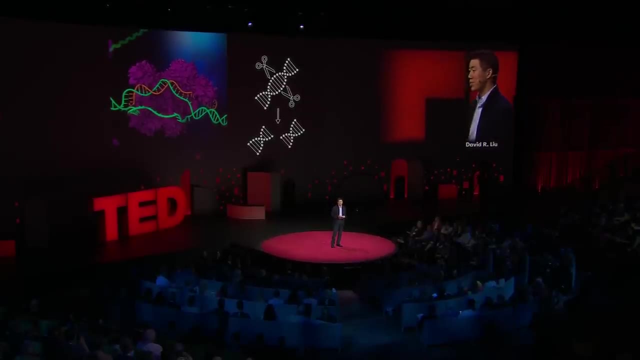 And the warhead in CRISPR is this purple protein that acts like molecular scissors to cut DNA, breaking the double helix into two pieces. If CRISPR couldn't distinguish between bacterial and viral DNA, it wouldn't be a very useful defense system. 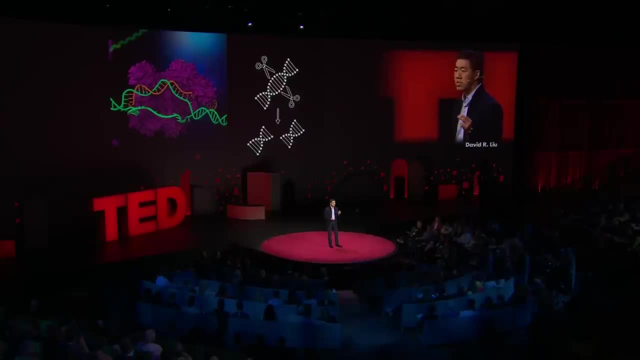 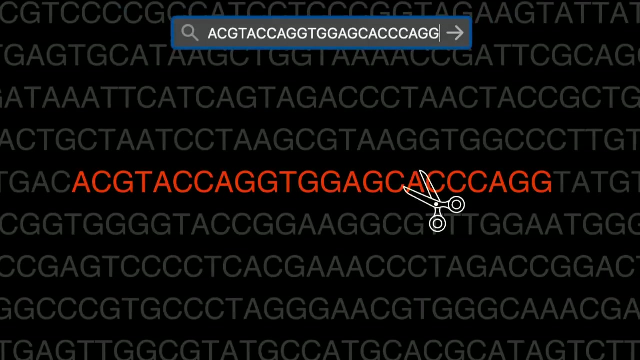 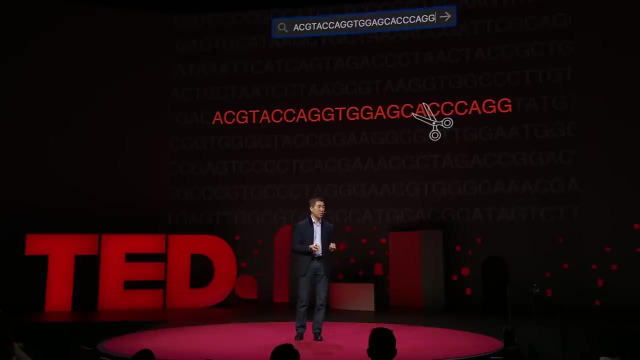 But the most amazing feature of CRISPR is that the scissors can be programmed to search for, bind to and cut only a specific protein, A specific DNA sequence. So when a bacterium encounters a virus for the first time, it can store a small snippet of that virus's DNA. 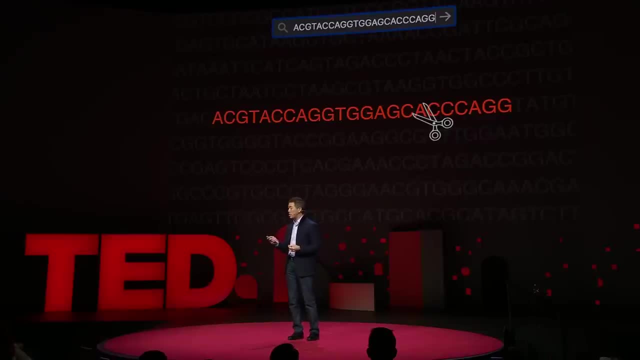 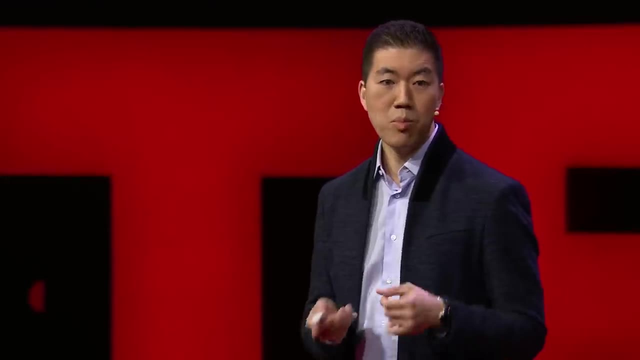 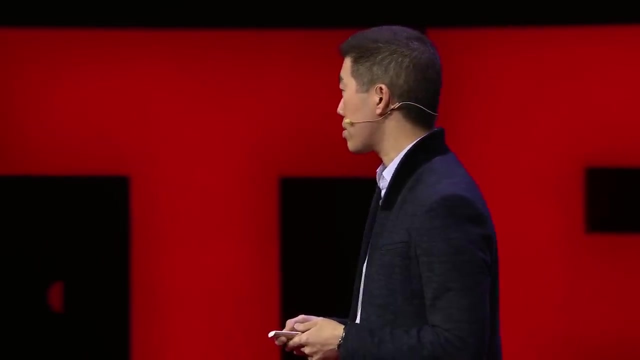 for use as a program to direct the CRISPR scissors to cut that viral DNA sequence during a future infection. Cutting a virus's DNA messes up the function of the cut viral gene and therefore disrupts the virus's life cycle. Remarkable researchers. 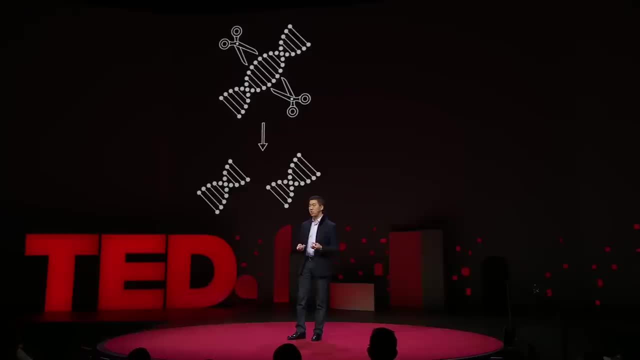 including in the United States, between Emmanuel Charpentier, George Church, Jennifer Doudna and Fun John, showed six years ago how CRISPR scissors could be programmed to cut DNA sequences of our choosing, including sequences in your genome, instead of the viral DNA sequences chosen by bacteria. 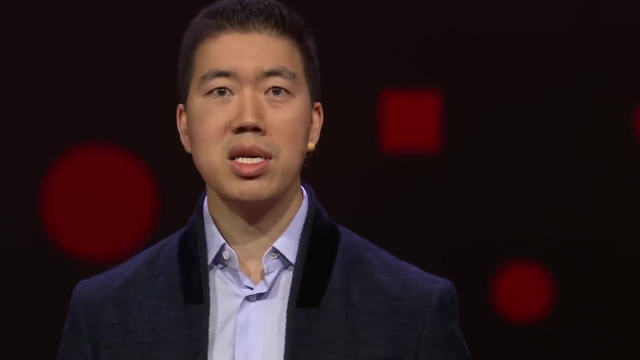 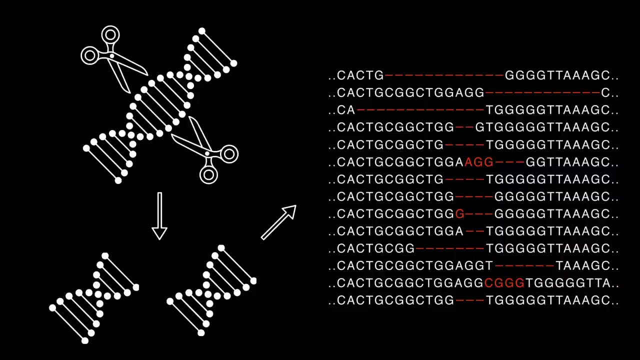 But the outcomes are actually similar. Cutting a DNA sequence in your genome also disrupts the function of the cut gene, typically by causing the infection, and by causing the infection and by the insertion and deletion of random mixtures of DNA letters at the cut site. 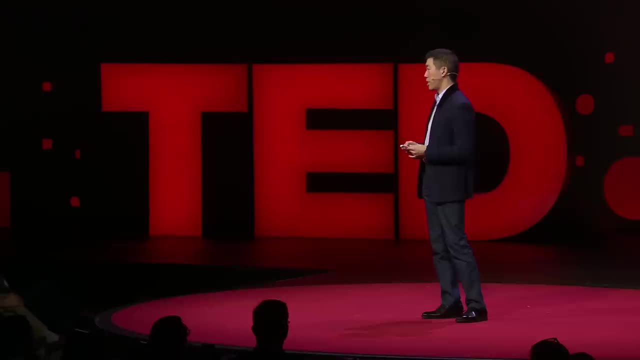 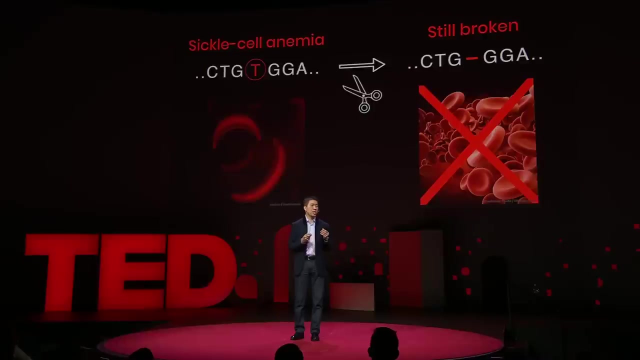 Now, disrupting genes can be very useful for some applications, But for most point mutations that cause genetic diseases. simply cutting the already mutated gene won't benefit patients, because the function of the mutated gene needs to be restored, not further disrupted. So cutting this already mutated hemoglobin. 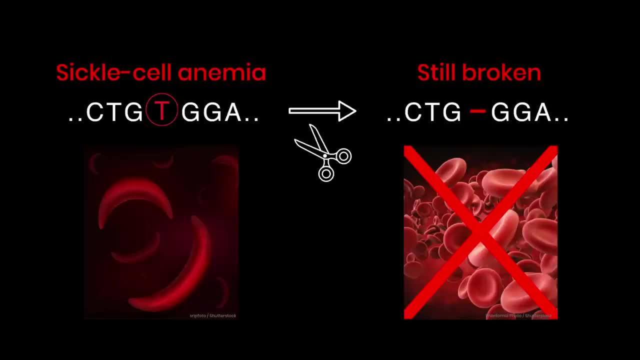 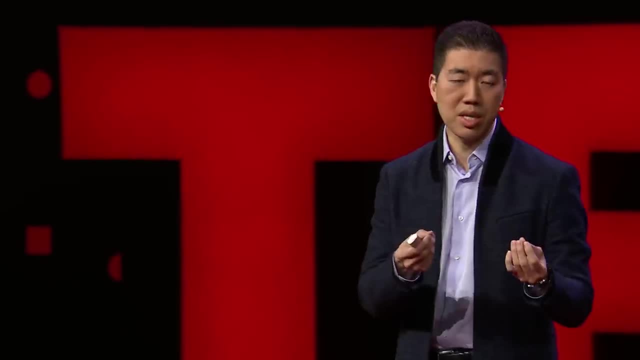 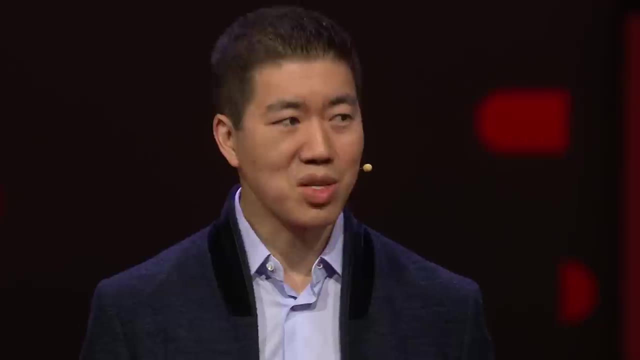 that causes sickle-cell anemia won't restore the ability of patients to make healthy red blood cells, And while we can sometimes introduce new DNA sequences into cells to replace the DNA sequences surrounding a cut site, that process unfortunately doesn't work in most types of cells. 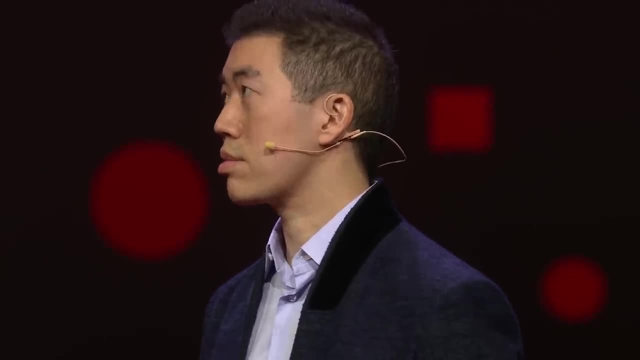 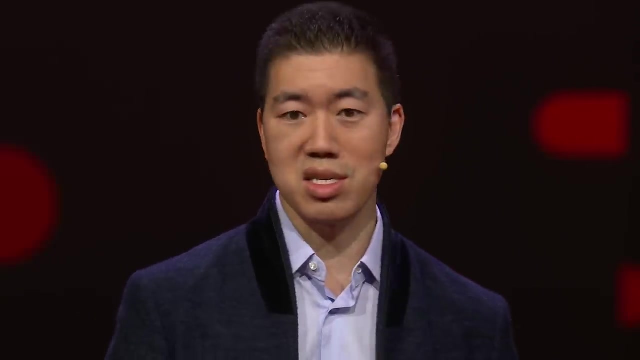 and the disrupted gene outcomes still predominate. Like many scientists, I've dreamed of a future in which we might be able to treat or maybe even cure human genetic diseases. But I saw the lack of a way to fix point mutations. 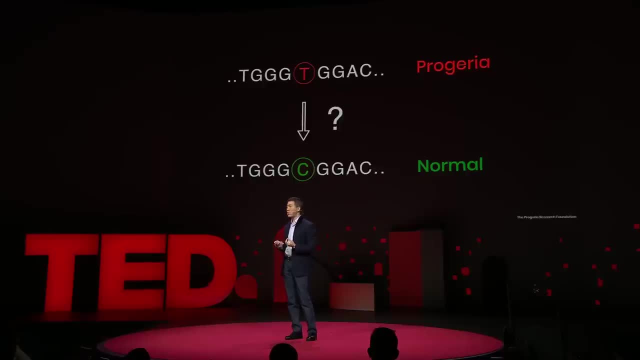 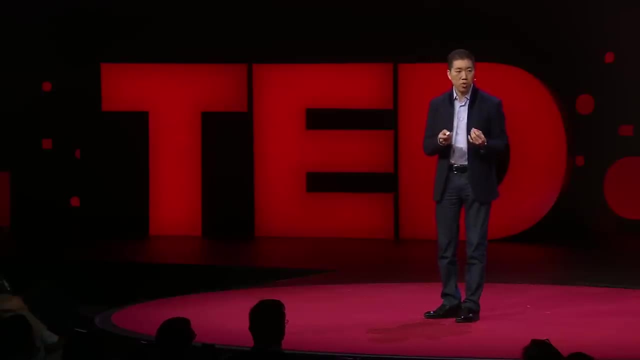 which cause most human genetic diseases, as a major problem standing in the way. Being a chemist, I began working with my students to develop ways on performing chemistry directly on an individual DNA base to truly fix, rather than disrupt, the mutations that cause genetic diseases. 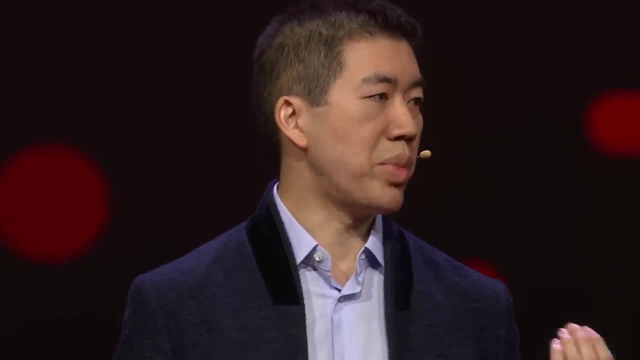 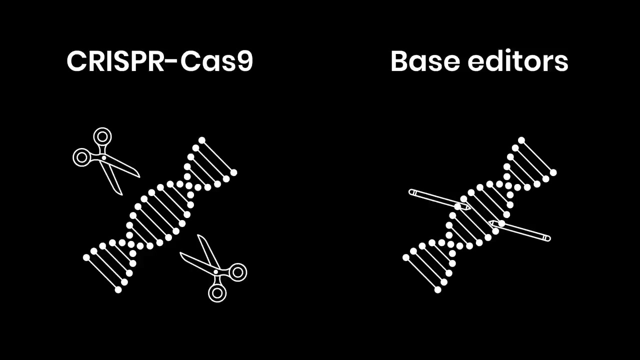 The results of our efforts are molecular machines called Base Editors. Base Editors use the programmable searching mechanism of CRISPR scissors, but instead of cutting the DNA, they directly convert one base to another base without disrupting the rest of the gene. So if you think of naturally occurring CRISPR proteins, 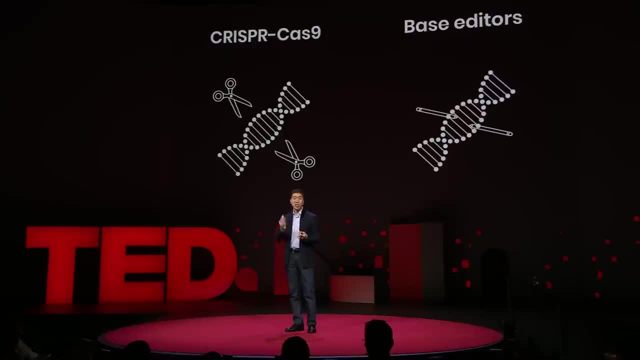 as molecular scissors. you can think of Base Editors as pencils capable of directly rewriting one DNA letter into another, by actually rewriting one DNA letter into another. So we can think of Base Editors as pencils capable of directly rewriting one DNA letter into another. 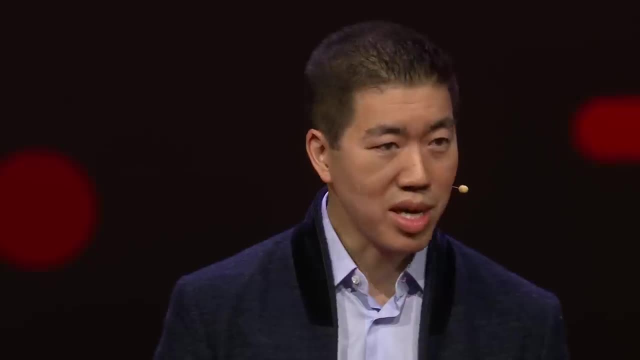 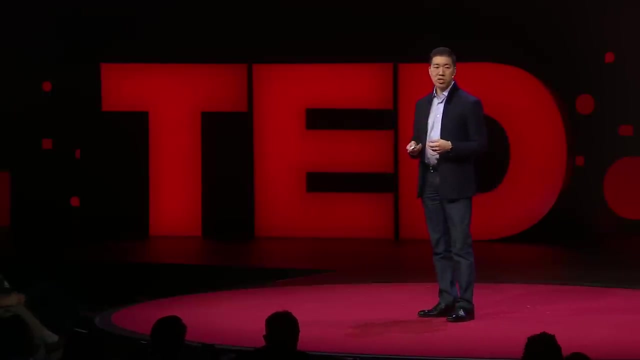 by actually rewriting one DNA letter into another, rearranging the atoms of one DNA base to instead become a different base. Now, base editors don't exist in nature. In fact, we engineered the first base editor shown here from three separate proteins that don't even come from the same organism. 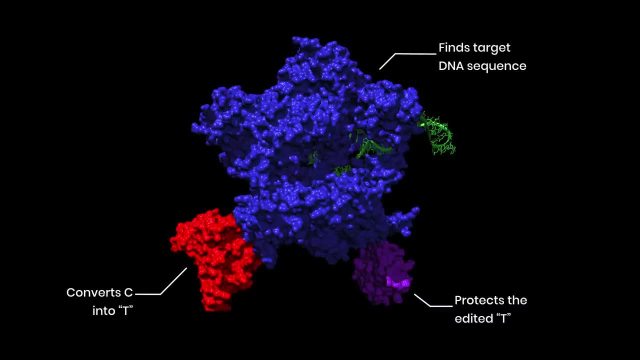 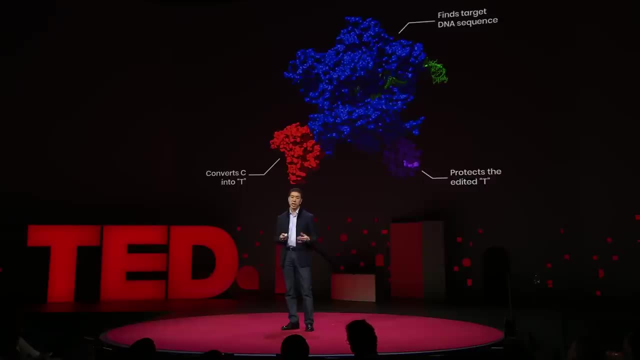 We started by taking CRISPR scissors and disabling the ability to cut DNA, while retaining its ability to search for and bind a target DNA sequence in a programmed manner. To those disabled: CRISPR scissors shown in blue. we attached a second protein in red. 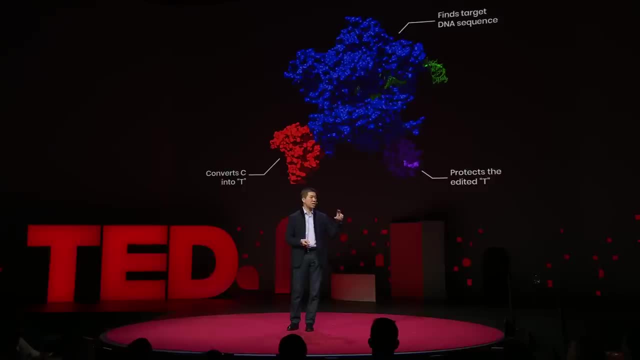 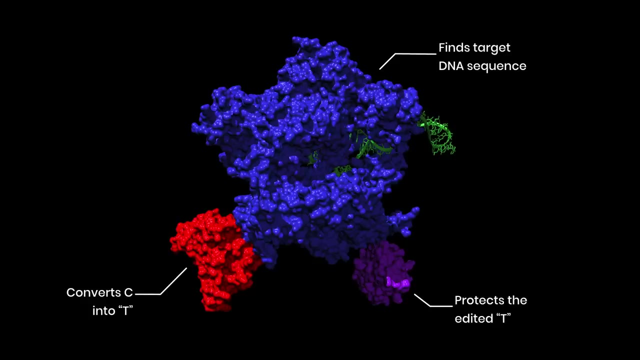 which performs a chemical reaction on the DNA base C, converting it into a base that behaves like tea. Third, we had to attach to the first two proteins the protein shown in purple, which protects the edited base from being removed by the cell. The net result is an engineered three-part protein. 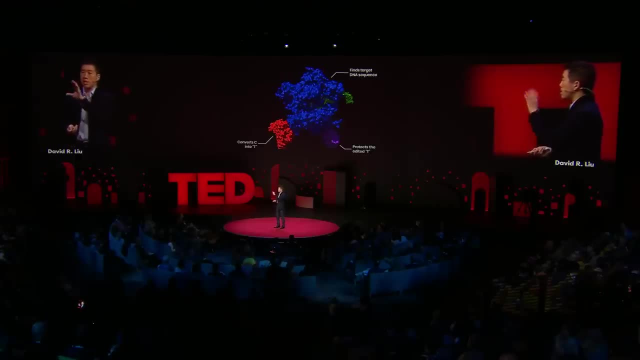 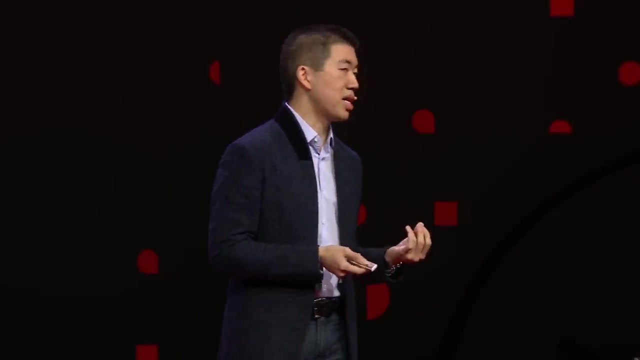 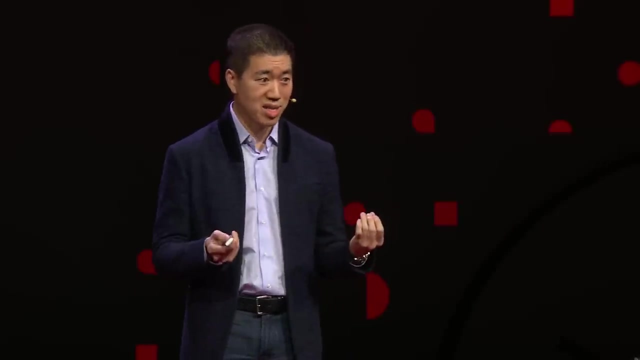 that, for the first time, allows us to convert Cs into Ts at specified locations in the genome. But even at this point our work was only half done, because in order to be stable in cells, the two strands of a DNA double helix have to form base pairs. 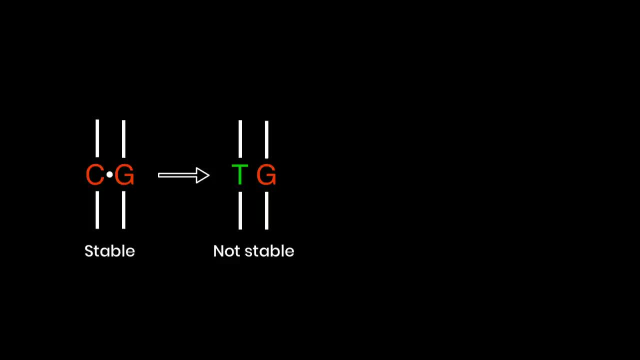 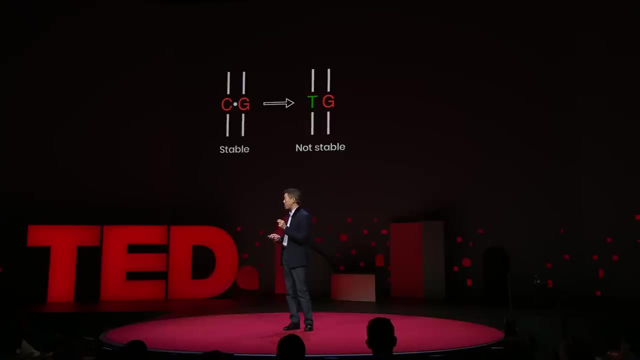 And because C only pairs with G and T only pairs with A, simply changing a C to a T on one DNA strand creates a mismatch, a disorganization. It's a disagreement between the two DNA strands that the cell has to resolve by deciding which strand to replace. 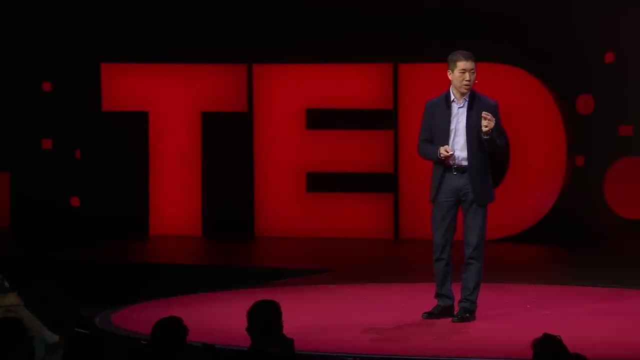 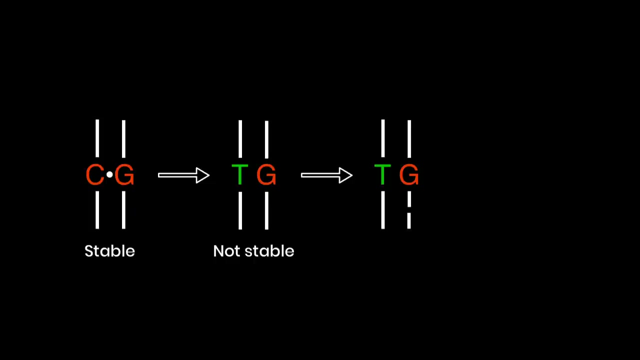 We realized that we could further engineer this three-part protein to flag the non-edited strand as the one to be replaced by nicking that strand. This little nick tricks the cell into replacing the non-edited G with an A as it remakes the nicked strand. 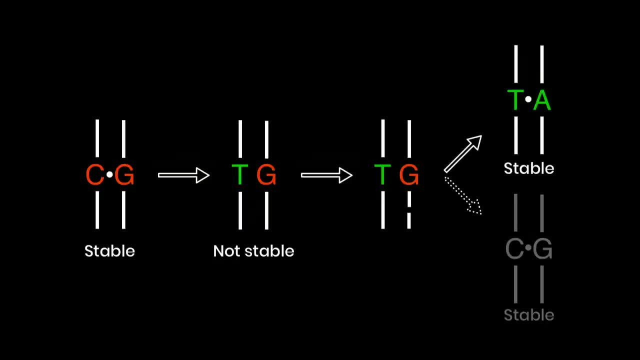 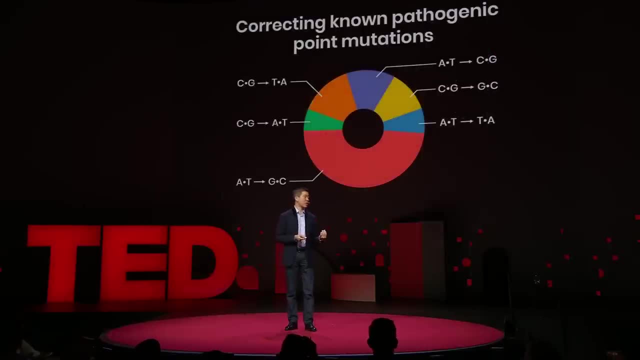 Thereby completing the conversion of what used to be a C-G base pair into a stable T-A base pair. After several years of hard work led by a former postdoc in the lab, Alexis Comor, we succeeded in developing this first class of base editor. 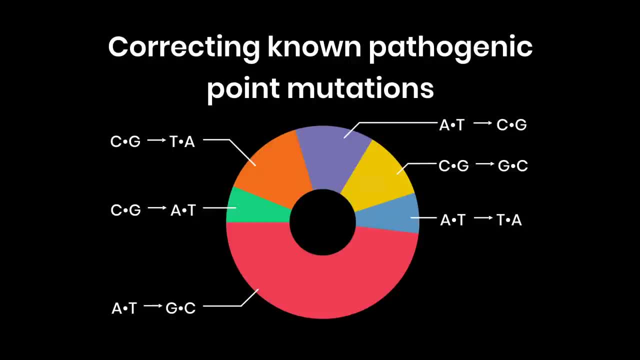 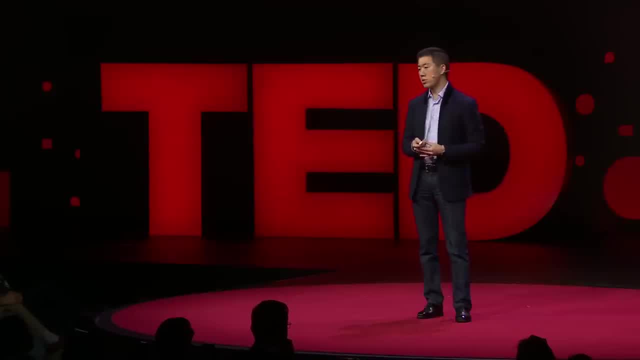 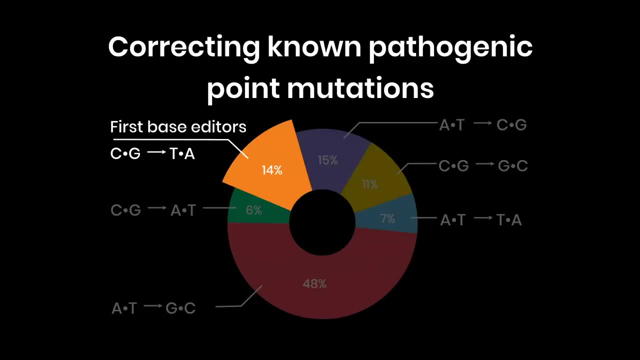 which converts Cs into Ts and Gs into As at targeted positions of our choosing. Among the more than 35,000 known disease-associated point mutations, the two kinds of mutations that this first base editor can reverse collectively account for about 14 percent. 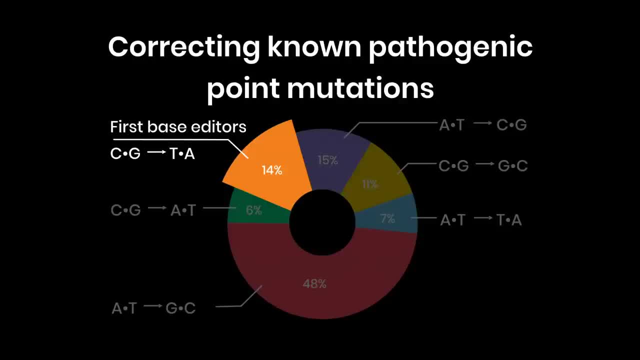 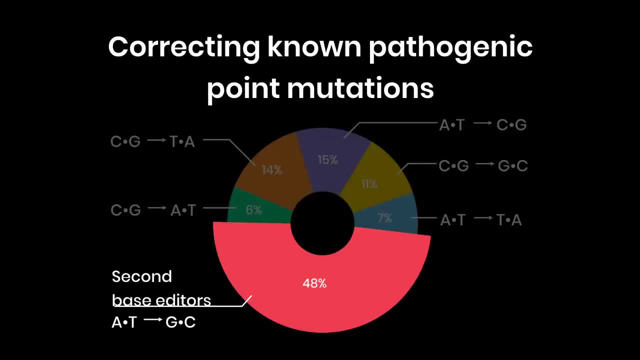 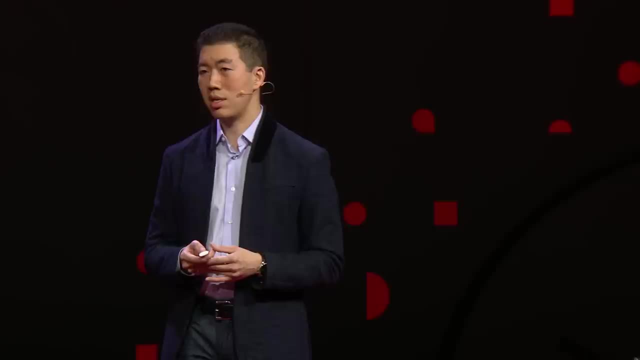 or 5,000 or so pathogenic point mutations, But correcting the largest fraction of disease-causing point mutations would require developing a second class of base editor, one that could convert As into Gs or Ts into Cs. Led by Nicole Godelli, a former postdoc in the lab, 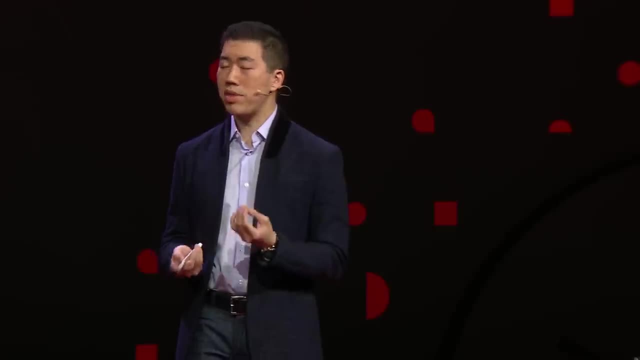 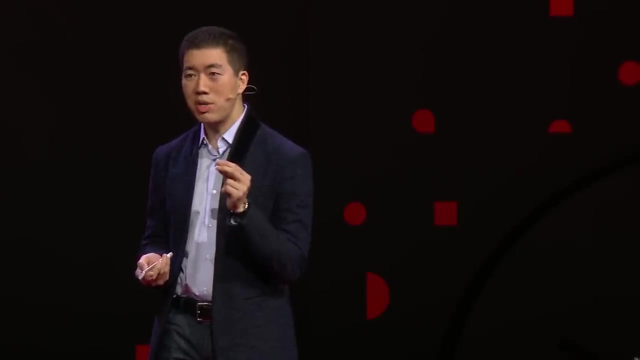 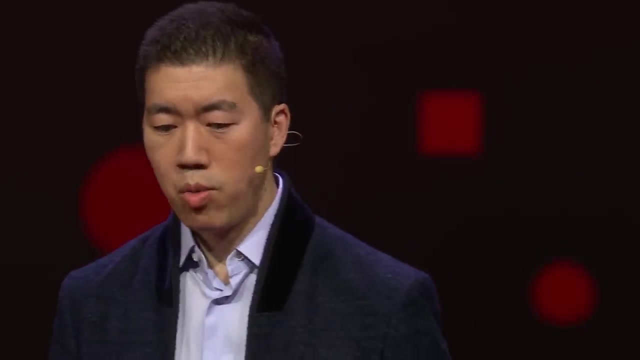 we set out to develop this second class of base editor, which in theory could correct up to almost half of pathogenic point mutations, including that mutation that causes the rapid aging disease, progeria. We realized that we could borrow once again the targeting mechanism of CRISPR scissors. 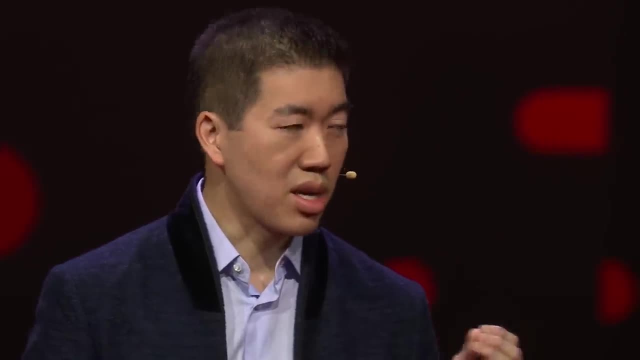 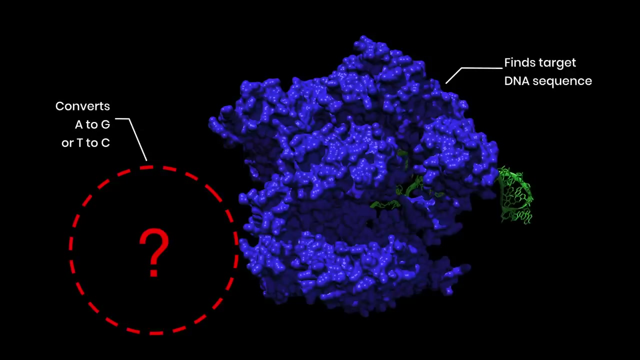 to bring the new base editor to the right site in a genome, But we quickly encountered an incredible problem. Namely, there is no protein that's known to convert A into G or T into C in DNA. Faced with such a serious stumbling block, 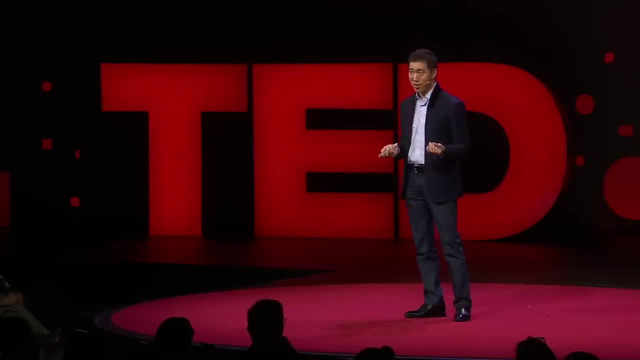 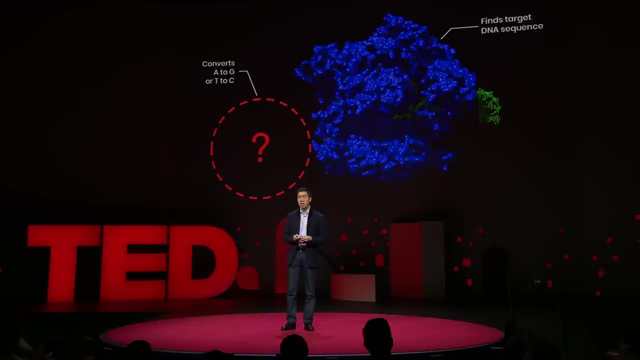 most students would probably look for another project, if not another research advisor, But Nicole agreed to proceed with a plan that seemed wildly ambitious at the time. Given the absence of a naturally occurring protein that performs the necessary chemistry, we decided we would evolve our own protein in the laboratory. 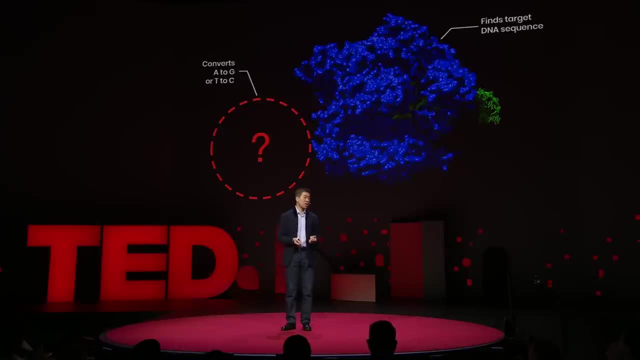 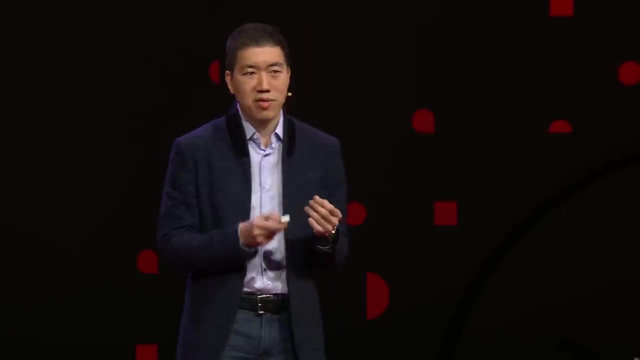 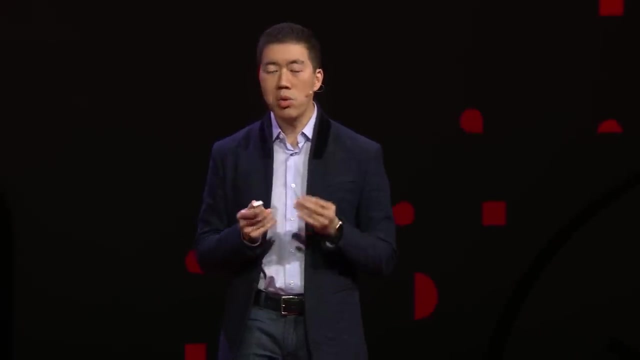 to convert A into a base that behaves like G, starting from a protein that performs related chemistry on RNA. We set up a Darwinian survival-of-the-fittest selection system that explored tens of millions of protein variants and only allowed those rare variants that could perform the necessary chemistry to survive. 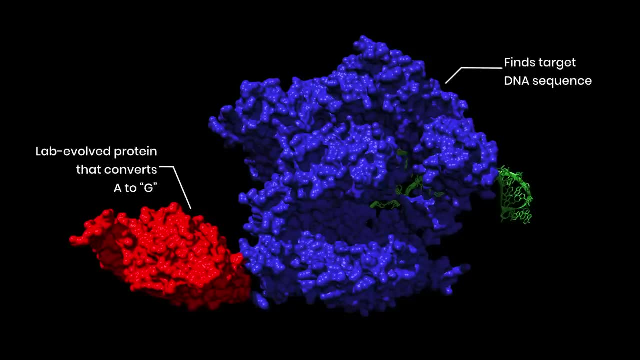 We ended up with a protein- shown here, the first- that can convert A in DNA into a base that resembles G, And when we attached that protein to the disabled CRISPR scissors shown in blue, we produced the second base editor, which converts As into Gs. 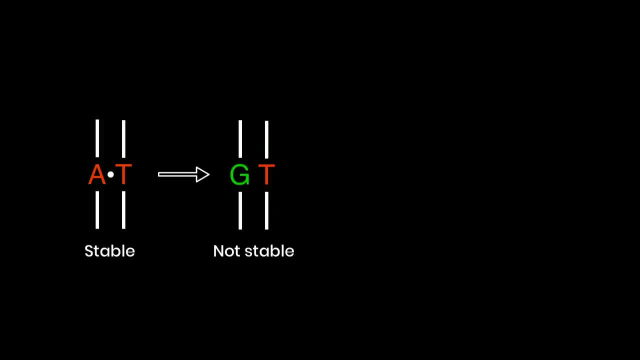 and then uses the same strand-nicking strategy that we used in the first base editor to trick the cell into replacing the non-edited T with a C, as it remakes that nicked strand, thereby completing the conversion of an A-T base pair to a G-C base pair. 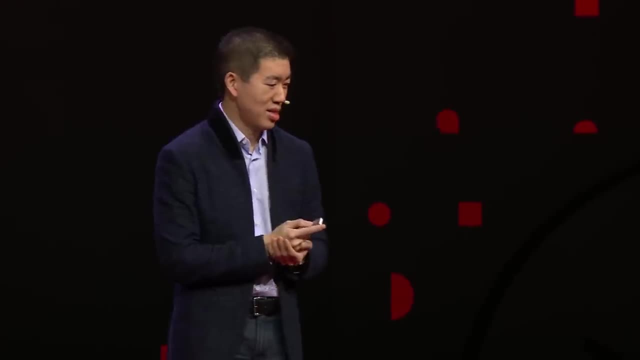 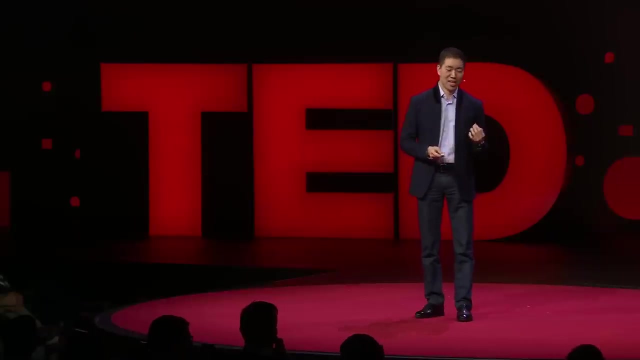 Thank you. As an academic scientist in the US, I'm not used to being interrupted by applause. We developed these first two classes of base editors only three years ago and one and a half years ago, But even that short time base editing has become widely used. 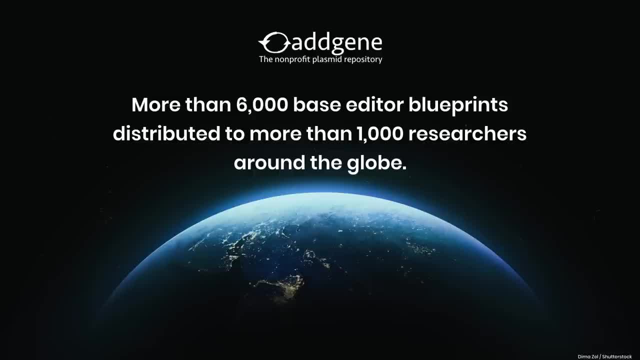 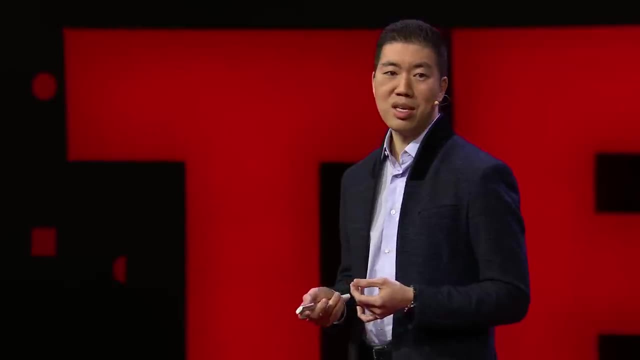 in the biomedical research community. Base editors have been sent more than 6,000 times at the request of more than 1,000 researchers around the globe. A hundred scientific research papers have been published already using base editors in organisms ranging from bacteria to plants, to mice, to primates. 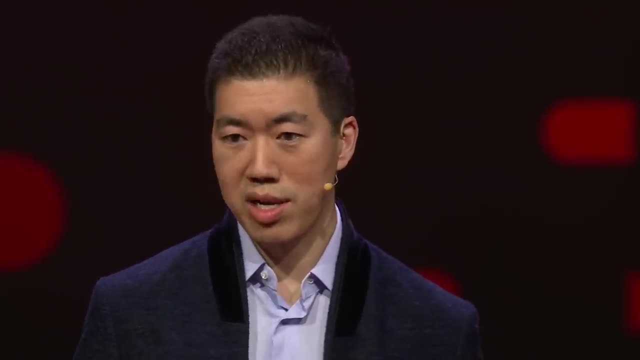 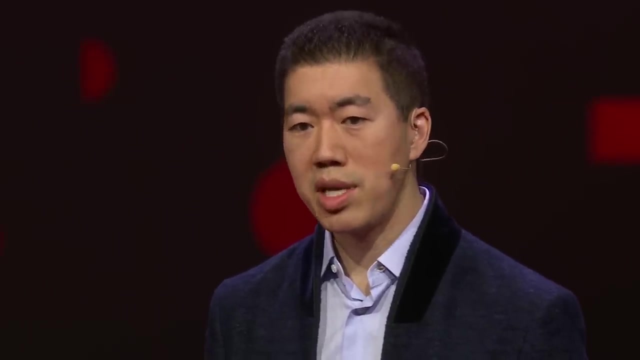 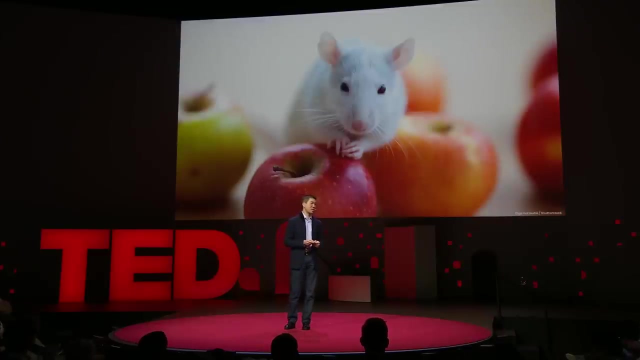 While base editors are too new to have already entered human clinical trials, scientists have succeeded in achieving a critical milestone towards that goal by using base editors in animals to correct point mutations that cause human genetic diseases. For example, a collaborative team of scientists led by Luke Koblen and John Levy 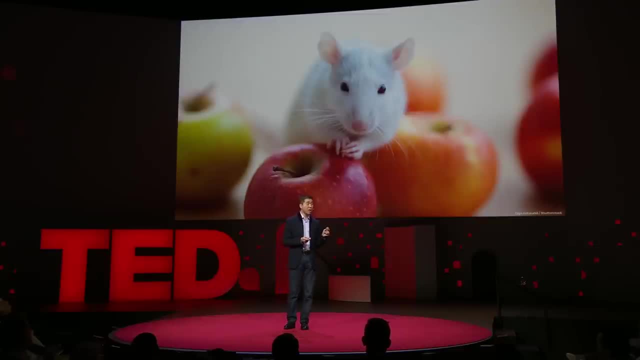 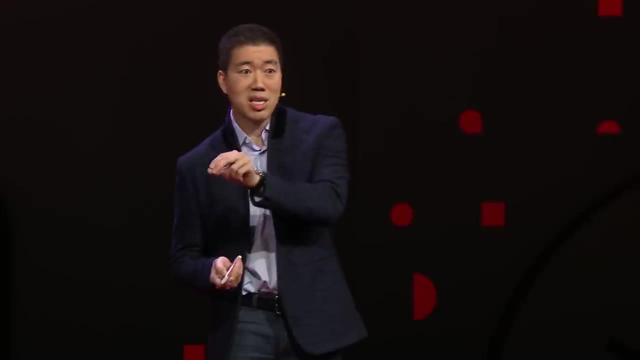 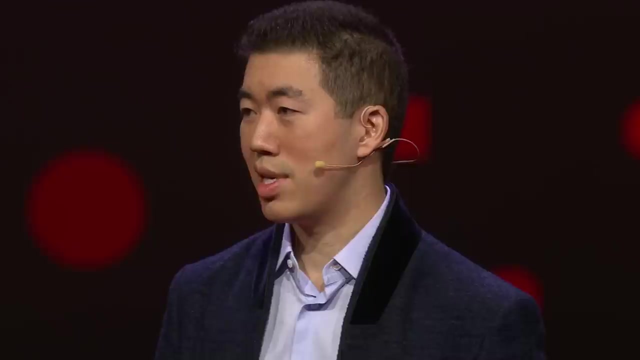 two additional students in my lab recently used a virus to deliver that second base editor into a mouse with progeria, changing that disease-causing T back into a C and reversing its consequences at the DNA, RNA and protein levels. Base editors have also been used in animals. 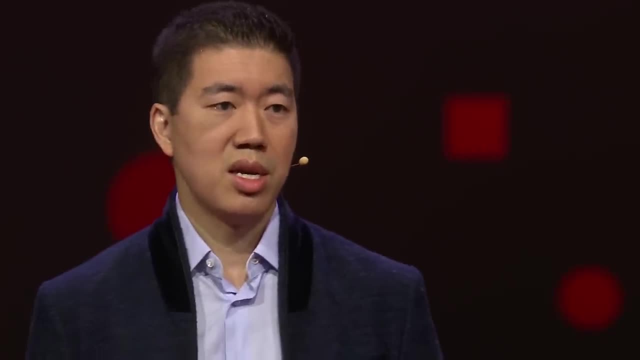 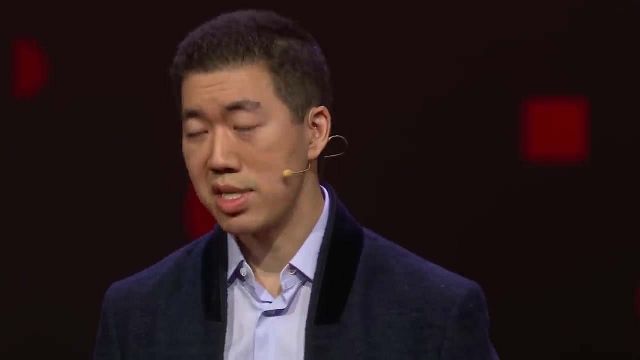 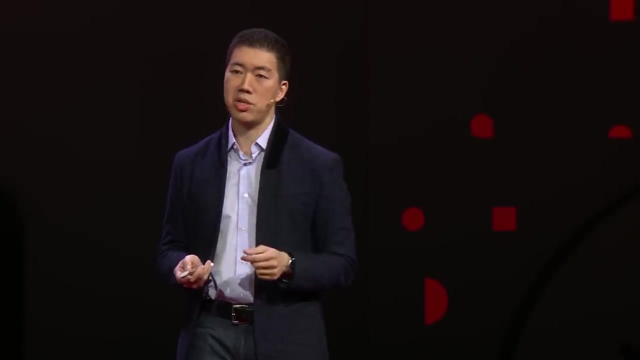 to reverse the consequence of tyrosinemia, beta thalassemia, muscular dystrophy, phenylketonuria, a congenital deafness and a type of cardiovascular disease, in each case by directly correcting a point mutation that causes or contributes. 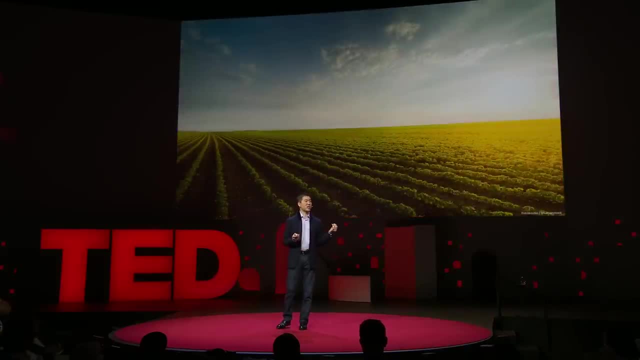 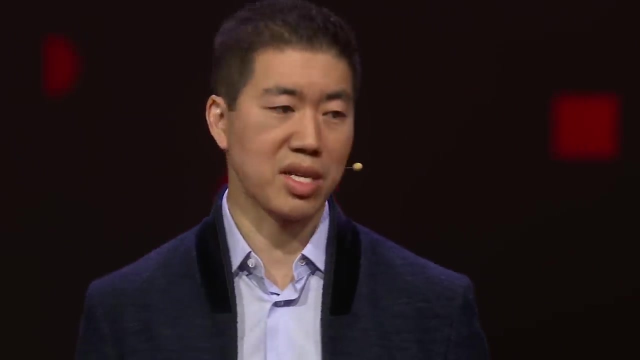 to the disease. In plants, base editors have been used to introduce individual single-DNA letter changes that could lead to better crops, And biologists have used base editors to probe the role of individual letters in genes associated with diseases such as cancer. Two companies I co-founded 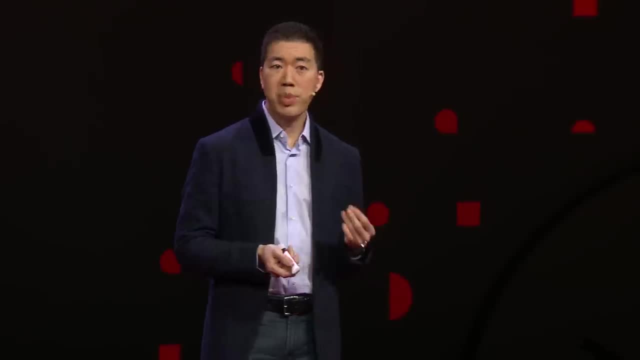 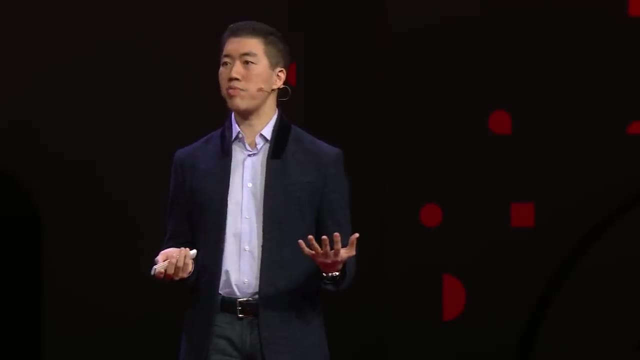 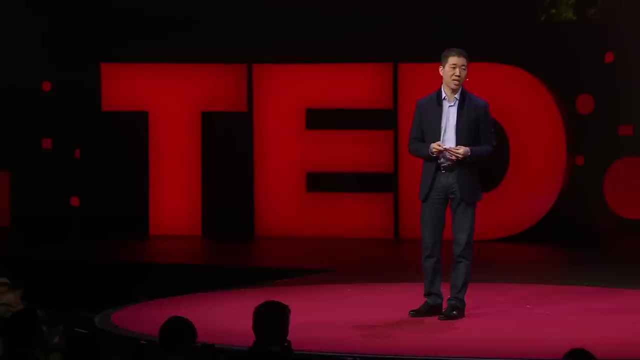 Beam Therapeutics and Pairwise Plants are using base editing to treat human genetic diseases and to improve agriculture. All of these applications of base editing have taken place in less than the past three years. On the historical timescale of science, the blink of an eye. 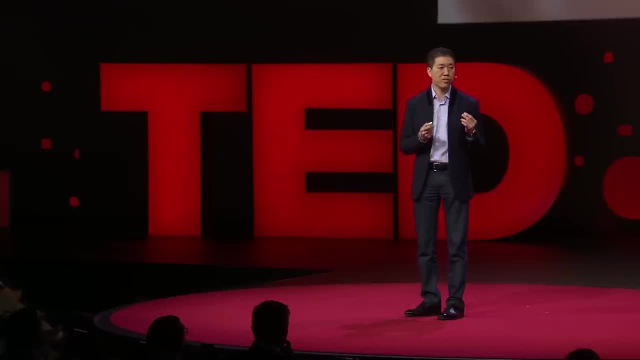 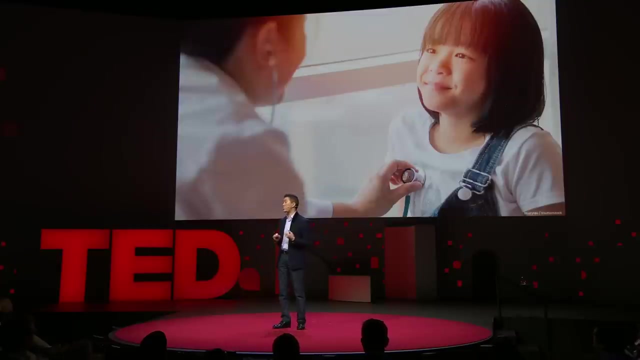 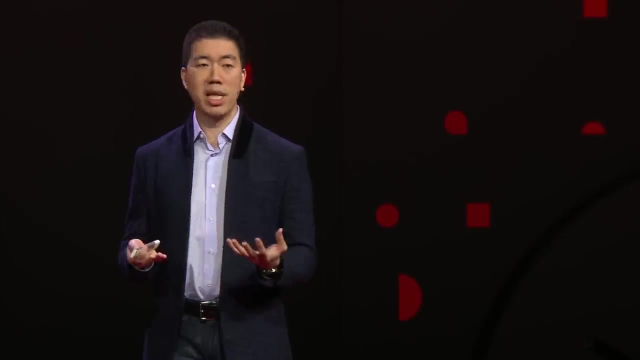 Additional work lies ahead before base editing can realize its full potential to improve the lives of patients with genetic diseases. While many of these diseases are thought to be treatable by correcting the underlying mutation in even a modest fraction of cells in an organ delivering molecular machines,